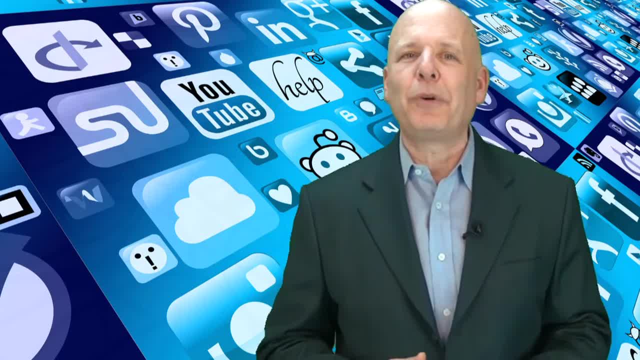 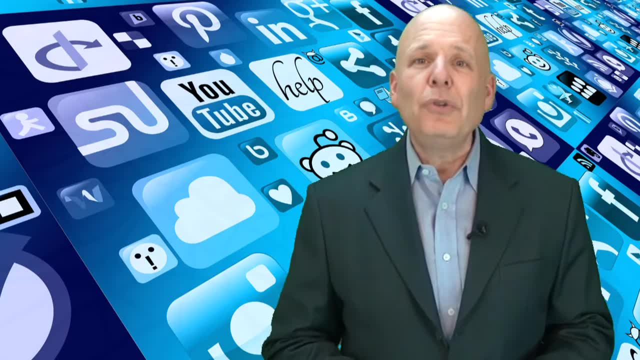 debacle. Now, is it just me? Well, as it turns out, most customers are maybe a little more tolerant than I am, but they still experience frustration. Facebook also polled 1,000 consumers on how long they were willing to wait when they connected. 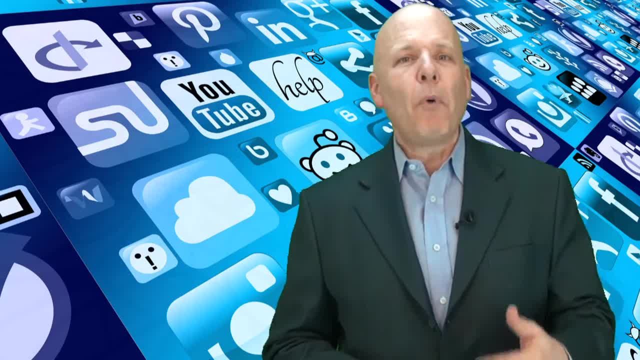 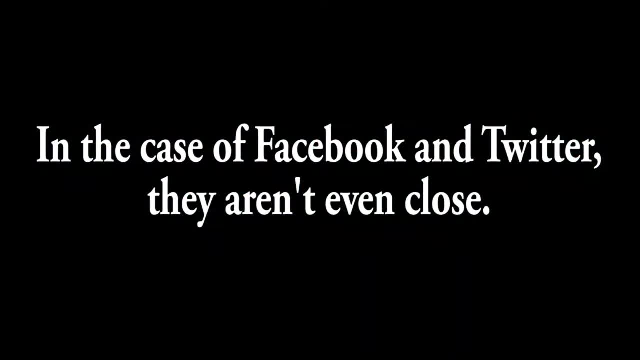 with the companies through these different channels. While most people are more accepting of the longer wait times, their patience doesn't last as long as the average company makes them wait. In the case of Facebook and Twitter, they aren't even close. 77% of consumers won't. 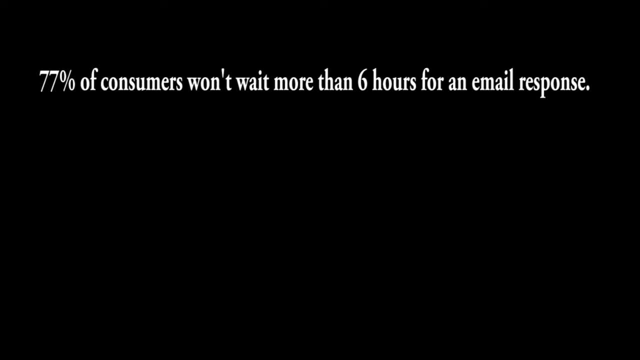 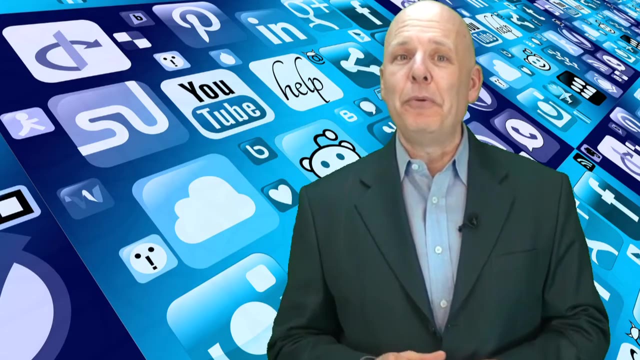 wait more than 6 hours for an email response. 85% of consumers using Facebook expect an answer within a day, Even 6 hours. 64% of consumers using Twitter expect a response time within an hour. All this looks like gloom and doom in the world of customer service, but there's good. 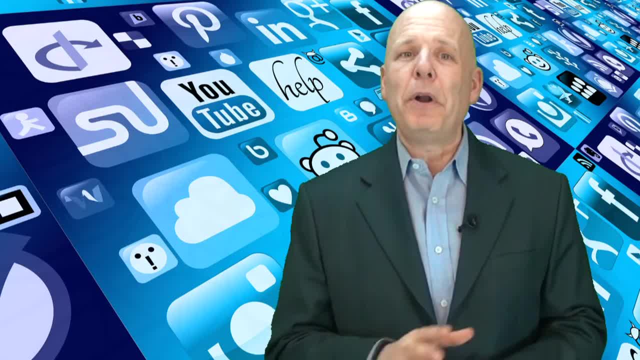 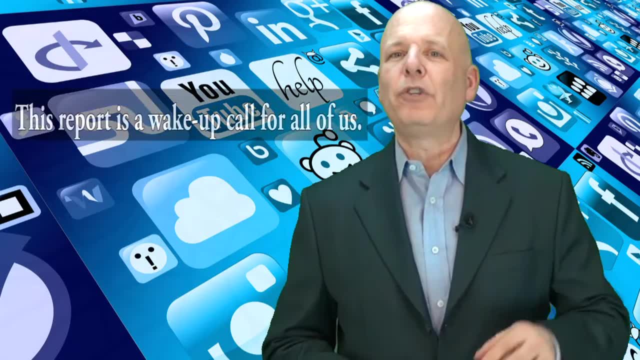 news. Yes, there are some rock stars out there who put others to shame. Some of these great companies respond within a minute or even less. But, more importantly, this report is a wake-up call for all of us. Quick response matters. Look at this report and determine. 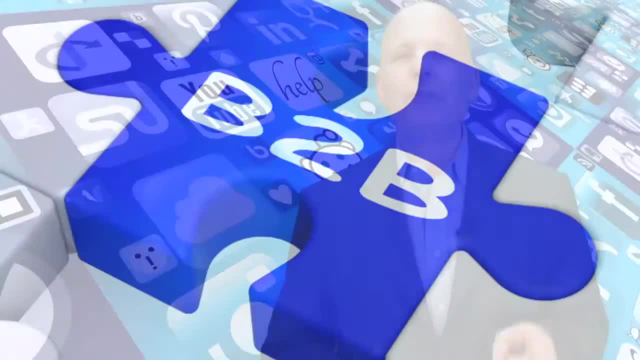 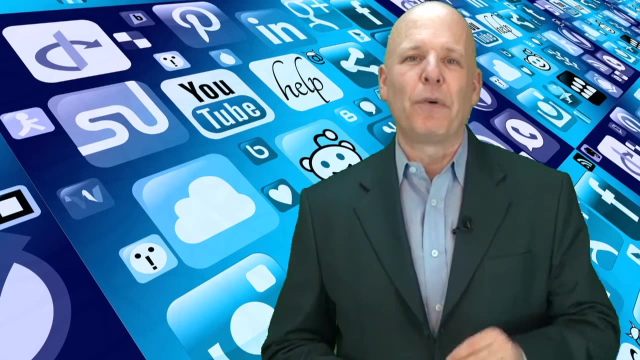 which industry you're in. If you feel that business-to-business doesn't apply, you're wrong. Regardless of the industry and the numbers, the concept of quick response is universal. When your customer has a question, they want an answer. When your customer has a problem, they want it resolved, And most 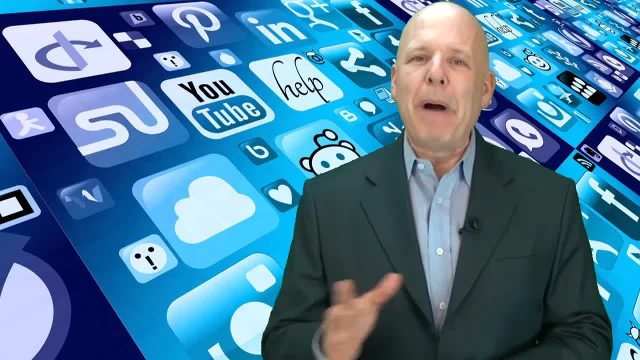 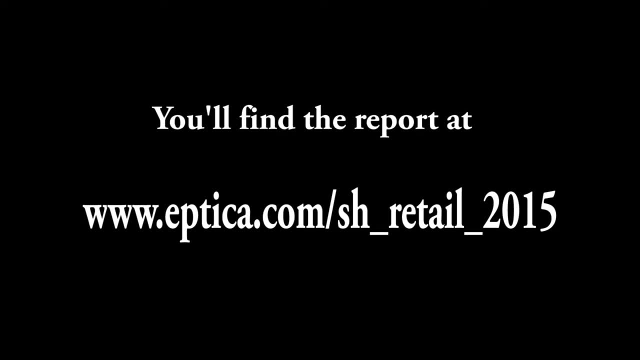 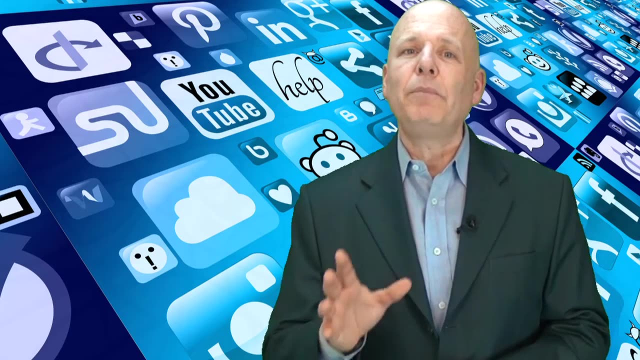 don't want to wait a day or two for you to get back to them. My suggestion is to take some action. First download the report- It's free- And then take a look at your response times And consider this, While the response times focus on outside. 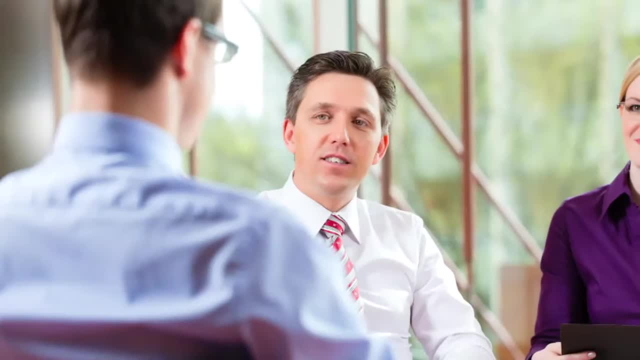 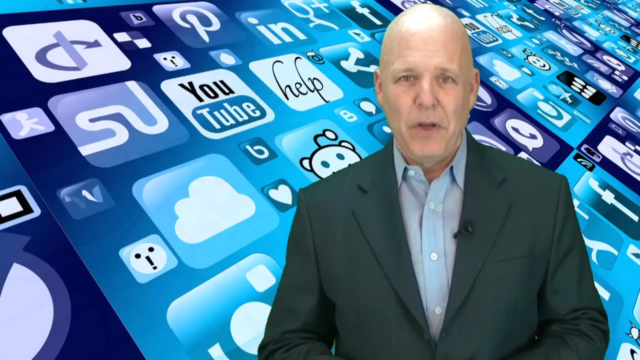 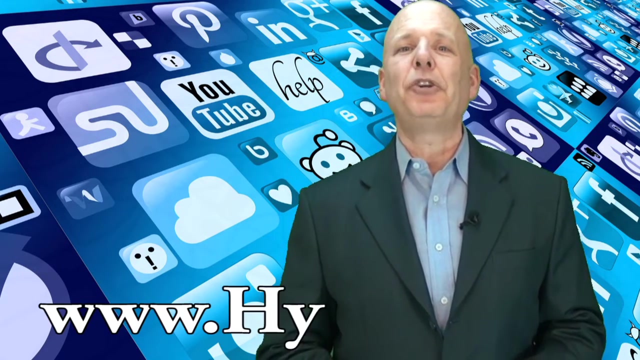 customers. how long do you take to respond to the people you work with, also known as your internal customers? Those are very important customers as well. Well, I hope you enjoyed this short lesson. Please be sure to visit my website, which is wwwhykencom. There you'll find more information about my speaking program and 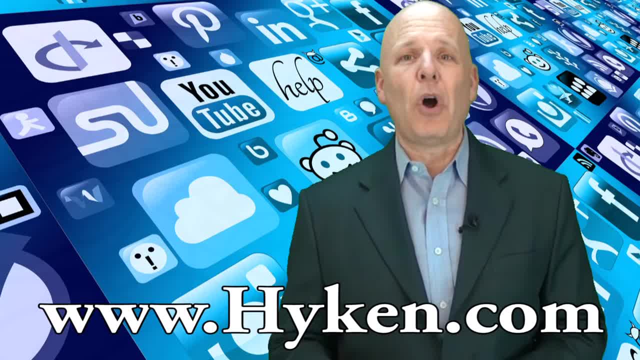 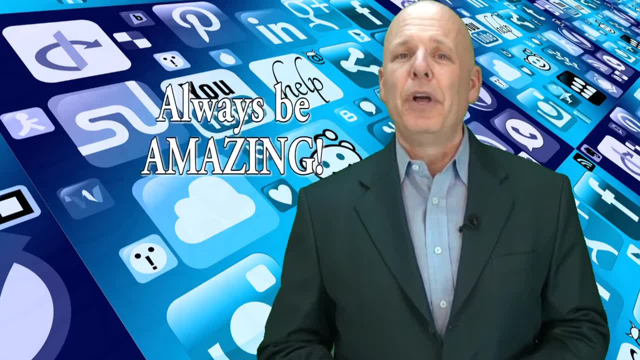 my website, wwwhykencom, As well as customer service articles that you can read and share with your colleagues. Thank you very much for tuning in. This is Shep Hyken reminding you to always be amazing.